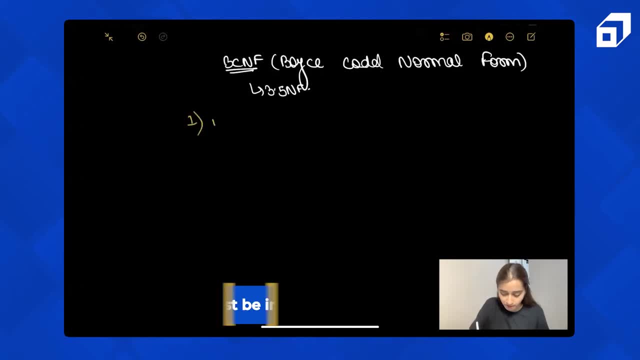 says that, of course, the first condition is it must be in 3NF. Okay, The second condition is: for all the functional dependencies from X to Y, X should be a prime region and that's it. So it's even more stricter than 3NF, Right? It just says that X should. 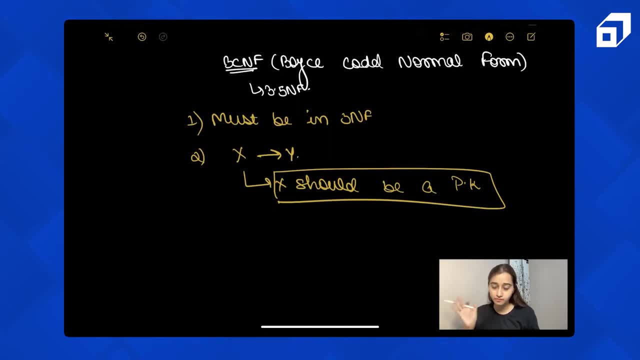 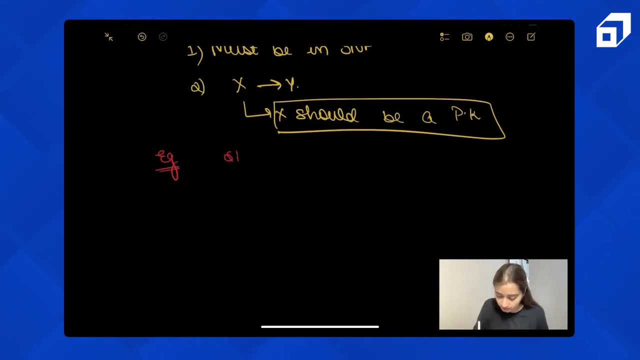 be in prime region. X should be a prime region. Okay, Again, let's understand with the help of an example. Let's take the normal, the example that we are taking The students. in the students table we have their ID, their name, their phone number and let's say their. 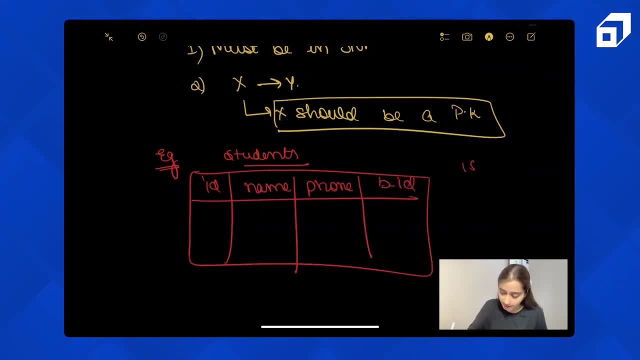 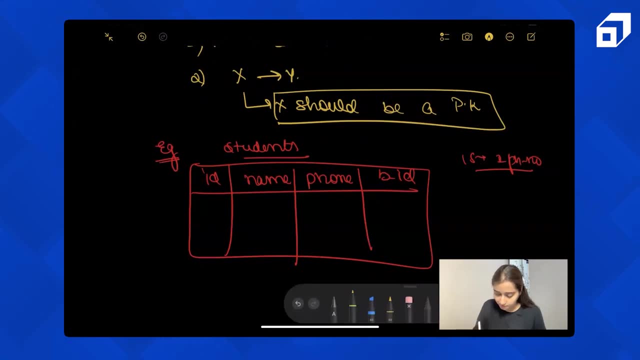 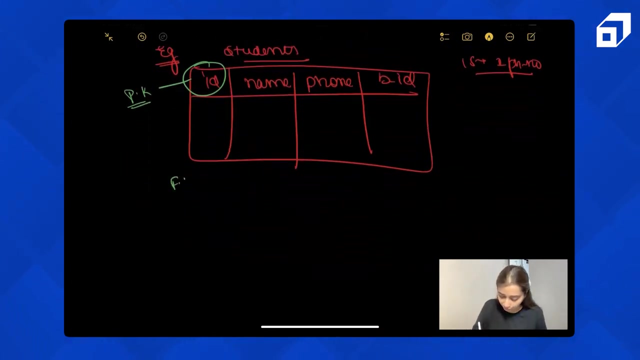 batch ID. Again, one student can have one phone number. Okay, First of all, the primary key of this table is ID. ID is the primary key of the table. Right Now let's write all the functional dependencies. The very first one is: 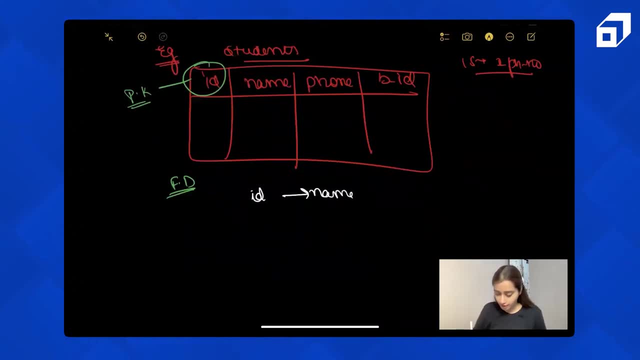 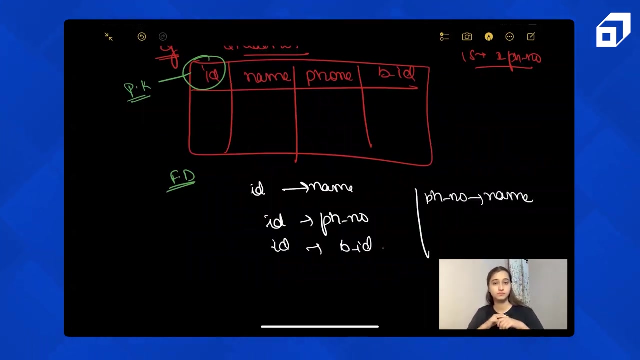 from ID. I can get their name From ID. I can get their phone number From ID. I can get their batch ID as well. Right Now, from phone number, can I get their name? Yes, because phone number is also unique. No two people, no two students, can have the same phone number. 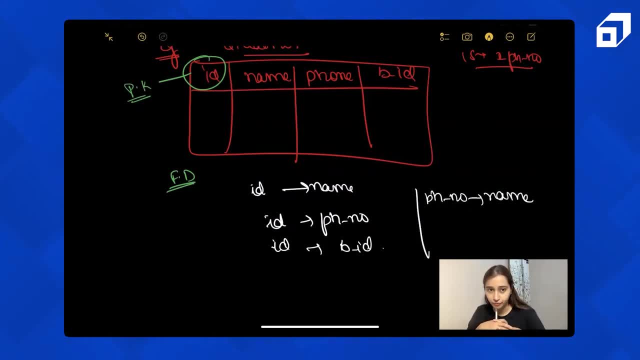 Right. First check if it is. if it is in 3NF, Okay, It's in 3NF because phone number is a part of a candidate key, Right, So it's in 3NF. Now comes BCNF. Is it in BCNF? No, Why? Because phone number is not a primary key And BCNF just say. 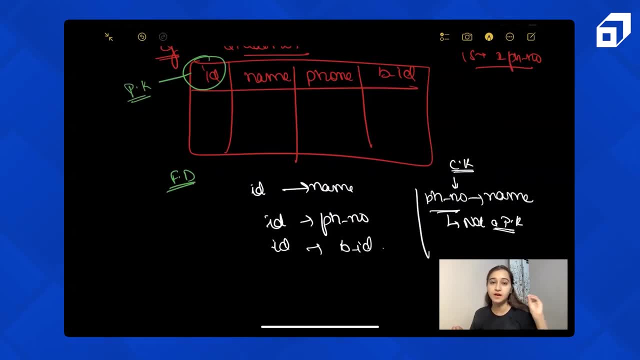 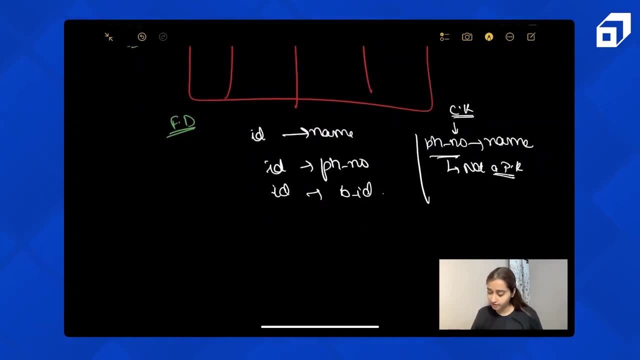 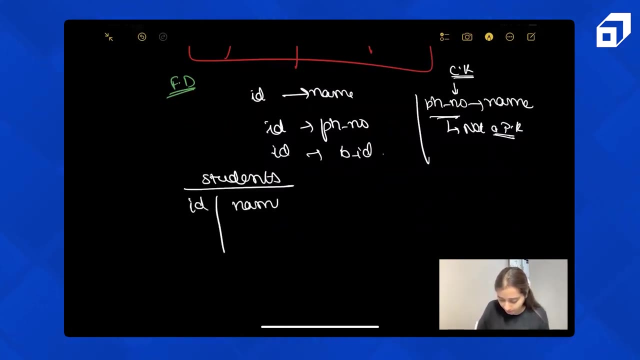 it's. it should be in primary key. It should be a primary key. So it's not a primary key, So it violates BCNF. Let's just normalize this, So one table we can have for students, their ID, their name and their. 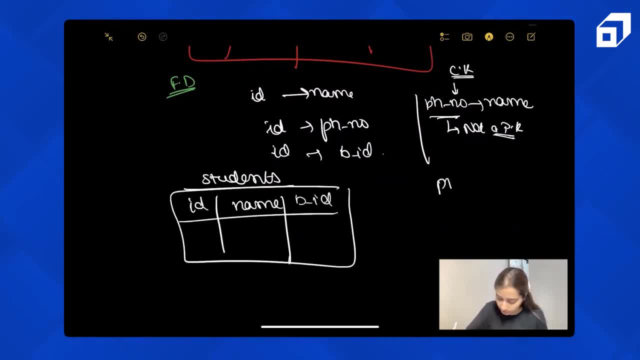 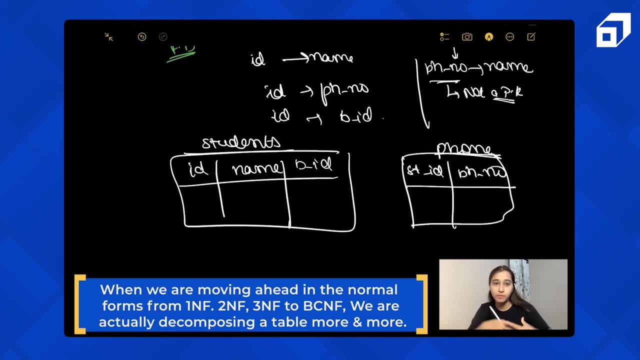 batch ID, One table for the phone number, In that we can have the student ID and we can have their phone number. Okay, So you are observing something When we are moving ahead in the normal forms from 1NF to 2 to 3 to BCNF. 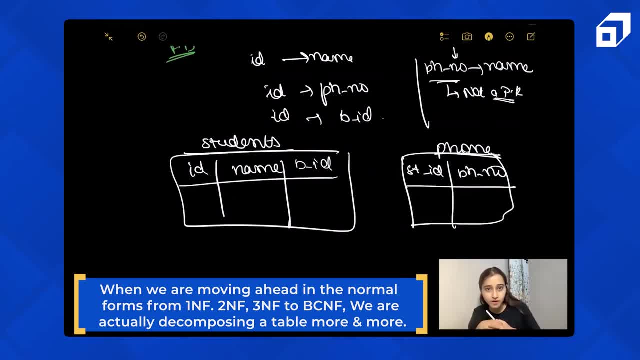 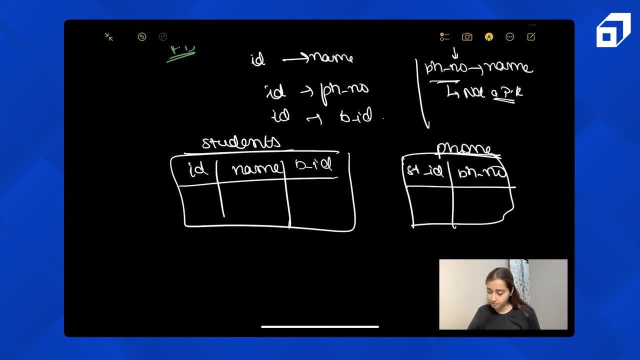 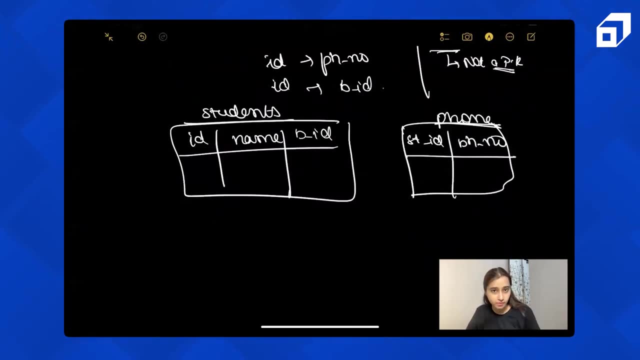 actually decomposing our table more and more right. so after that, after 3nf, bcnf, practically it's not used because we are actually doing more harm than good when we have to do some query on our table right, when we have to join our table right, the wastage of memory is there. so after: 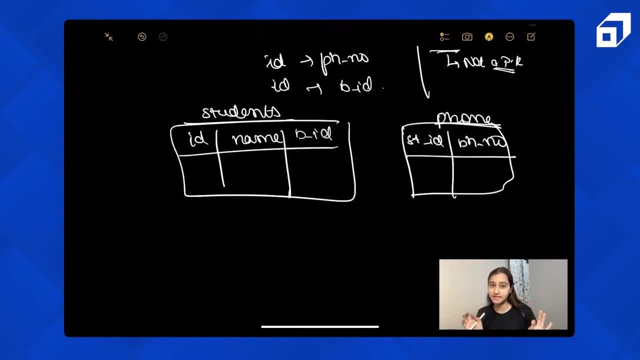 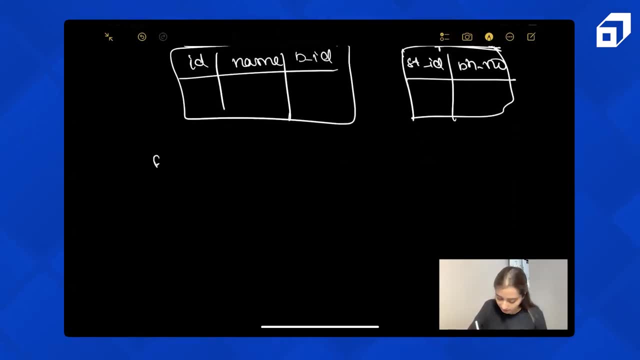 that practically it's not used. so till 3b, cnf. only you need to know about right. so let's again take an example. take example 2 for bcnf. let's take a relation- a, b, c, d, e. given to you right and functional dependencies as a to b, c and c to b. the very first thing is you have to check. 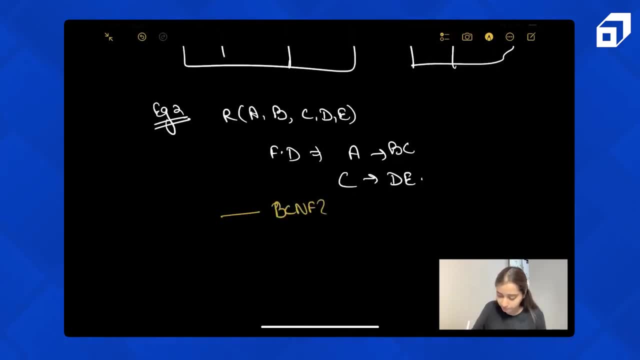 is it in bcnf or not? if it is not, you have to convert it. right, let's check that. first we need to find the primary key of the stable. so primary key can be: pause the video. try to solve it on your own, okay. so primary key is a. can a be the primary key? from a i can get bc, and from c i can get d, e as well. 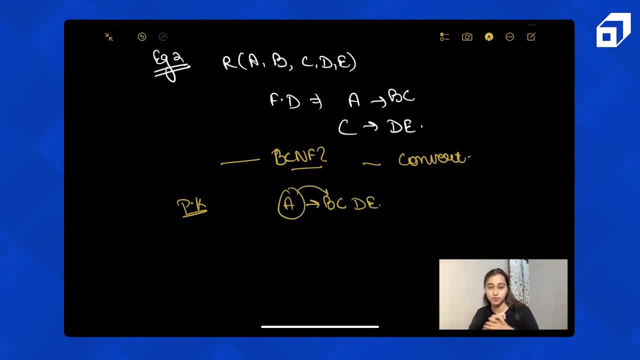 so from a i am getting all the other attributes, all the other columns of the table. from b, can i get anything? no, from c can i get? yeah, i can get d, e, but after that no other attributes, no other columns. right? so a becomes my primary, the very 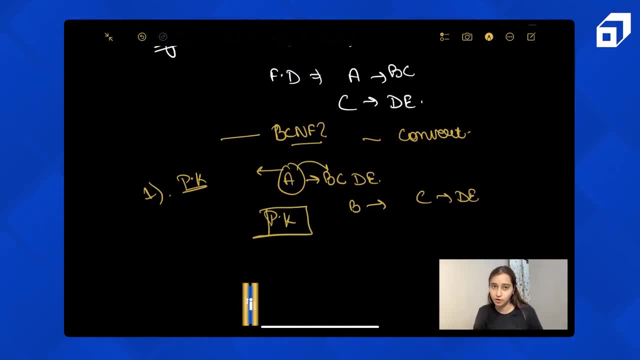 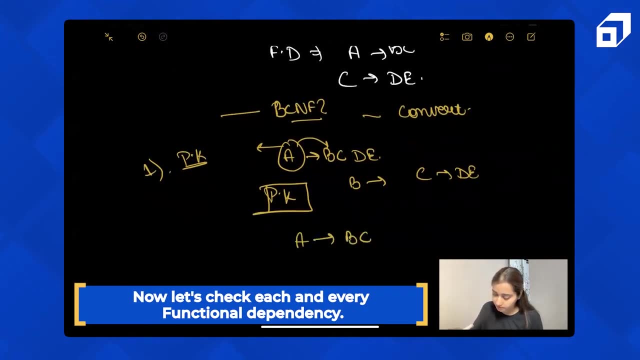 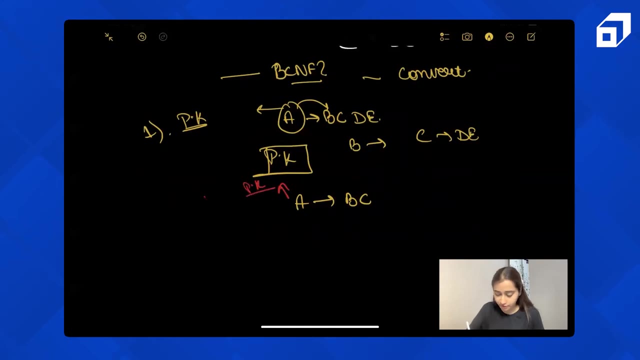 first step is to find the primary key, so a becomes my primary key of the table. clear now let's check for each and every functional dependence. the very first one is a to b c. a to b c. now a is a primary key, so it follows b, c and f right now. the next functional dependency is c to d, e. 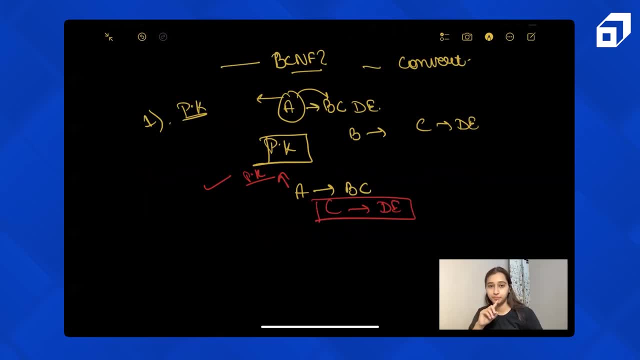 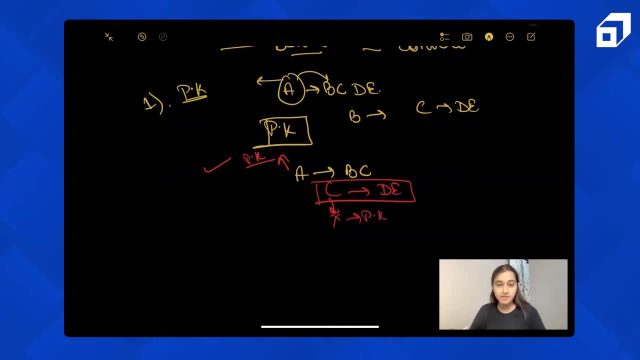 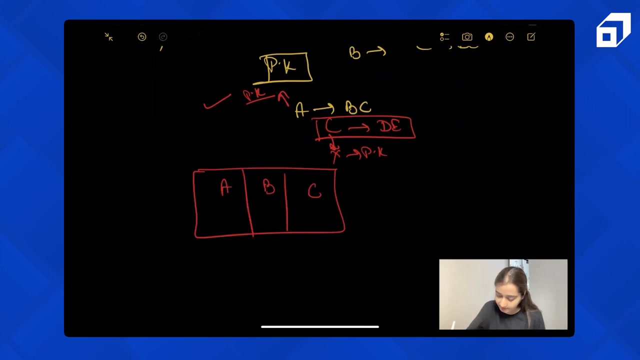 now it follows b, c and f. no, because it just says that this x should be a primary key, but c is not a primary key, so it violates b, c and f. so we have to normalize it. to normalize it, let's decompose our dependencies. the very first table can be now a, b, c. second table can be c, d and e. 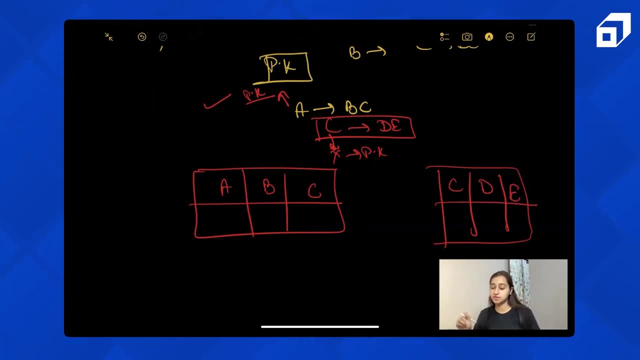 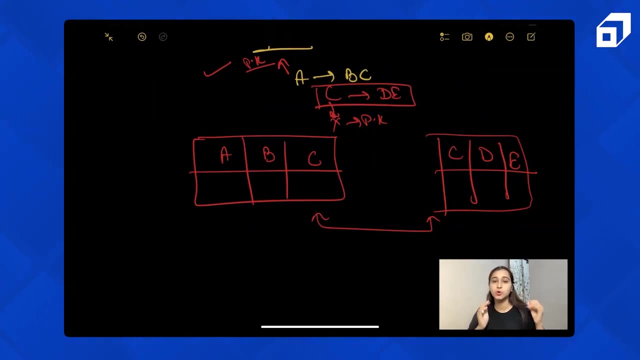 okay, so this is the decomposed table, so that's pretty much all about. we need to know, uh in about normal forms, about normalization, okay, so now let's time to revise it. revise all the concepts that we have learned, and i'll give you some examples of the concepts that we have learned, and i'll give you some examples of the. 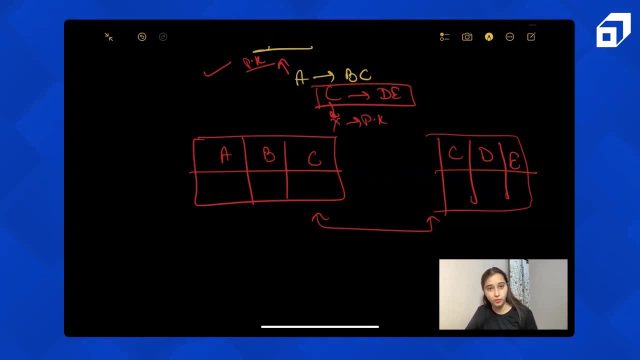 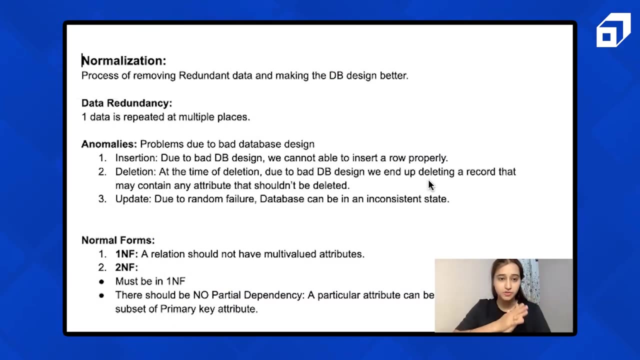 concepts that we have learned, and i'll give you some examples, also some table or some functional dependencies to solve on your own, okay. so, yeah, let's revise this. so let's quickly revise whatever we have learned about normalization, okay. so normalization is, it's a process of removing read and repetitive data and making the database design better. 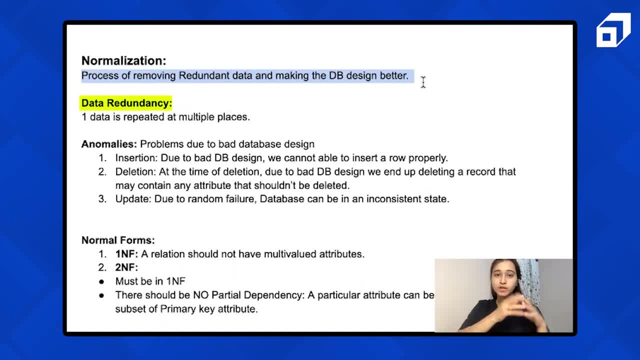 okay, that's the main function of normalization. now, what is data? redundancy means one number of data has repeated at multiple places. now redundant data can also replace the overwhelm data, create many problems, many problems. that is anomalies. they are called anomalies problems due to bad database design. the very first problem is insertion, at the time of inserting something. 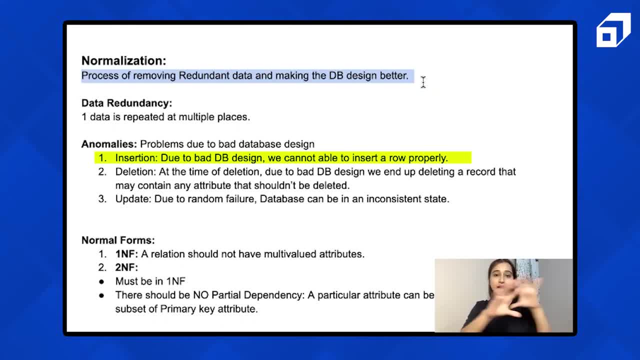 due to bad database design, you cannot able to insert that row properly. you want to insert something, but due to bad database design, due to redundancy, you can't able to insert that row properly. okay, then, deletion at the time of deletion: due to bad database design, we end up. 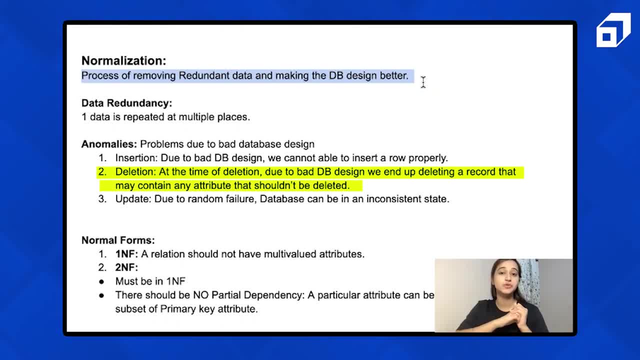 deleting a record that may contain any attribute that shouldn't be deleted. okay, update anomaly: due to random failure, your database can be in an inconsistent state. so update anomaly means due to bad database design, maybe your database is in an inconsistent state. okay, it's not consistent anymore. 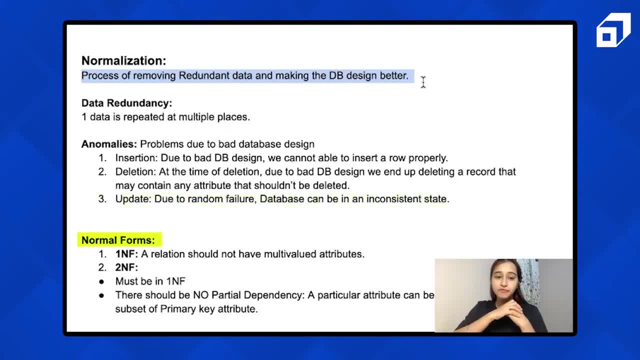 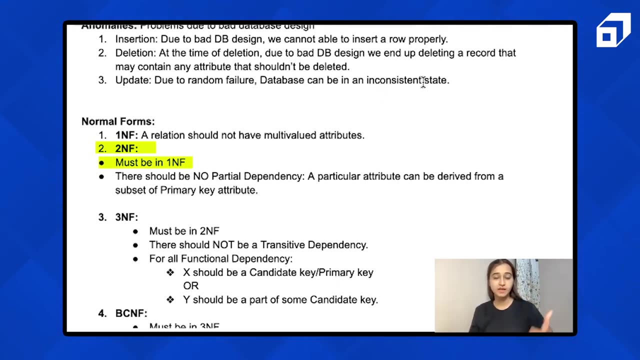 now normal forms. normal forms: the very first one is 1nf. a relation should not have multi-valued attributes. that's it. it's the easiest form. it just says your attribute should be single value: 2nf first. it follows 1nf second. there should be no partial dependency. partial dependency means 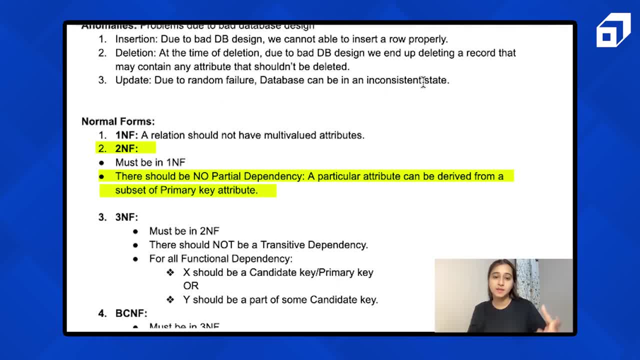 a particular attribute can be derived from a subset of primary key attribute. if let's say ab is a particular attribute, then it should be a subset of primary key attribute. if let's say primary key b is d is derived from b. so this is partial dependency, because d is derived from a. 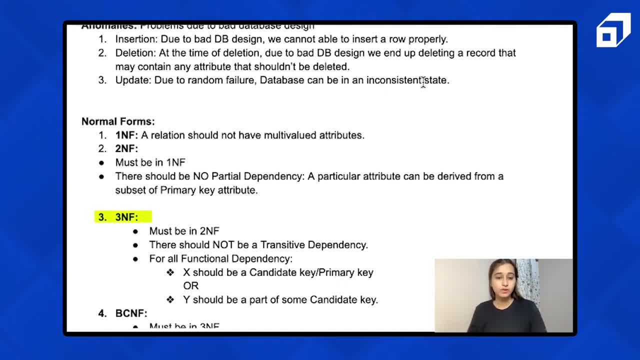 partial of the key, now 3 and f first. it must follow 2 and f then there should not be a transitive dependency. transitive dependency means if a drives b, b drives c, it implies that a drives c that shouldn't be there, or for all functional dependency. the one is x should be a candidate. 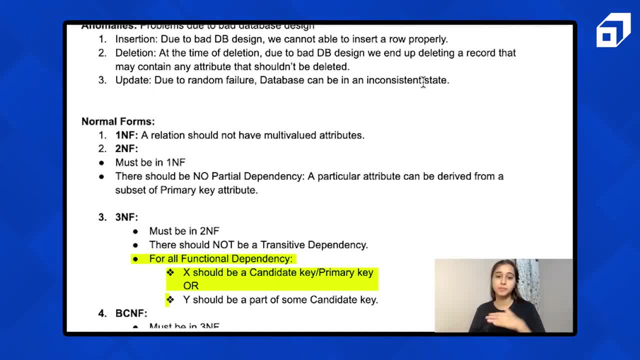 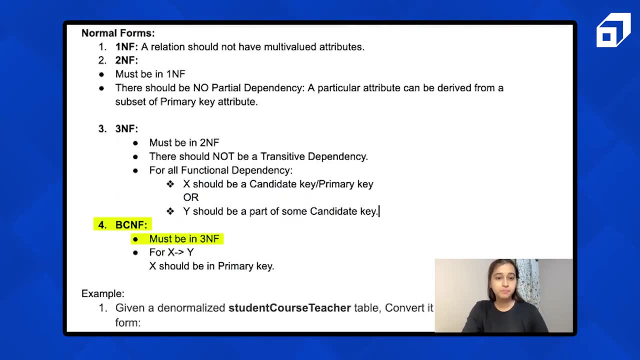 key, or a primary key, or y should be a part of some candidate. so either of the two conditions. true, then that means it's in 3 and f. okay now b, c and f. it's a stricter form, stronger form of 3 and f. it says that for x to y, x drives y, x should be in primary key. that's it. 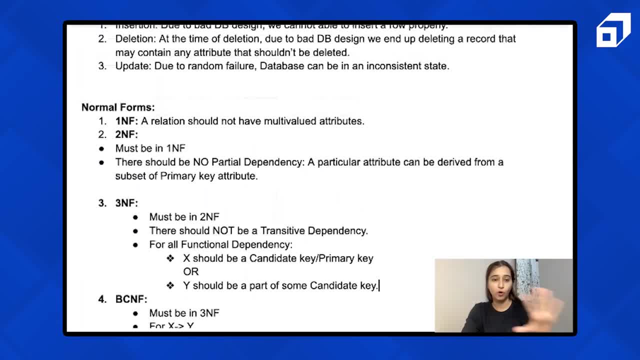 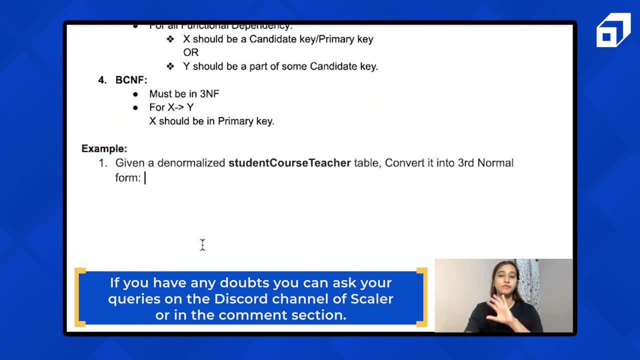 you okay. now these are all the normal forms and about all the normalization. now these are some of the examples. you have to solve it. if you have any doubts, you can ask your query in the discord channel of scalar and you can ask the queries in comment section also. 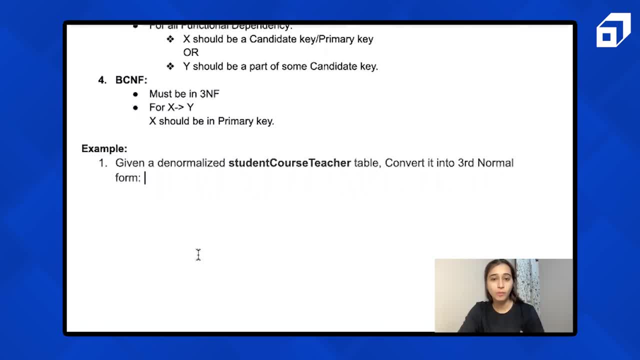 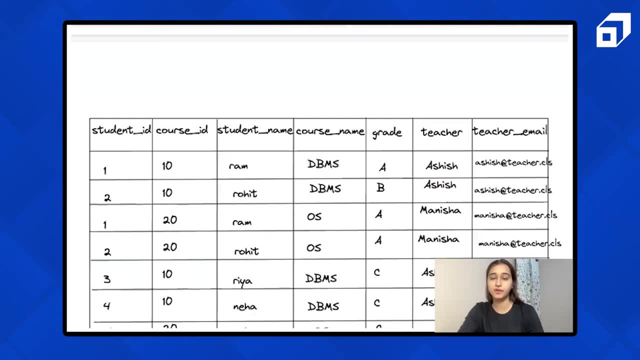 so okay. so very first one is: you are given a denormalized student course teacher table. you have to convert it into third normal form. okay, first check. if it is in third normal form, no need to convert. if it is in third normal form, no need to convert. if it is in third normal form. 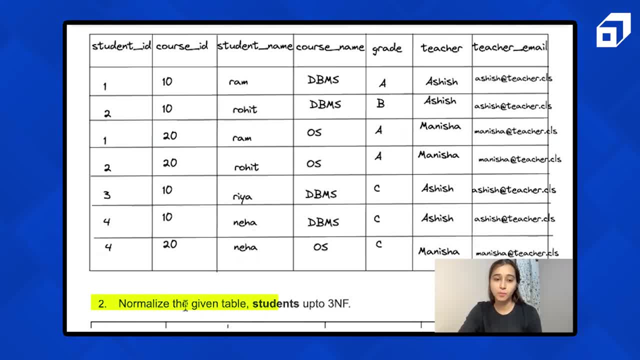 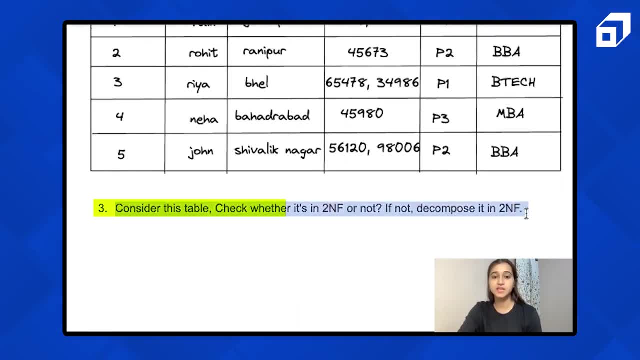 if it is not, you have to normalize it. second question: you have to normalize the table, students up to 3n, up to 3n, if you have to check it. third one is: you have to consider this table and check whether it's in 2nf or not, or if it's not. you have to decompose, you have to normalize.